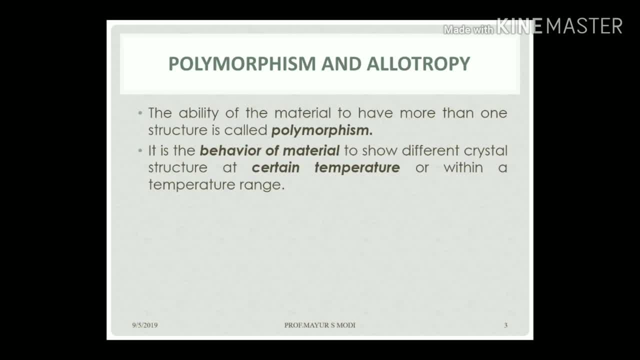 structures at the certain temperatures or within a temperature range. it means what? at different temperature, material having a different structure, and structure is directly related to the properties of the material. so different temperature having a different property of the materials. the atomic arrangement may be changed according to the change in temperature. such a change in a 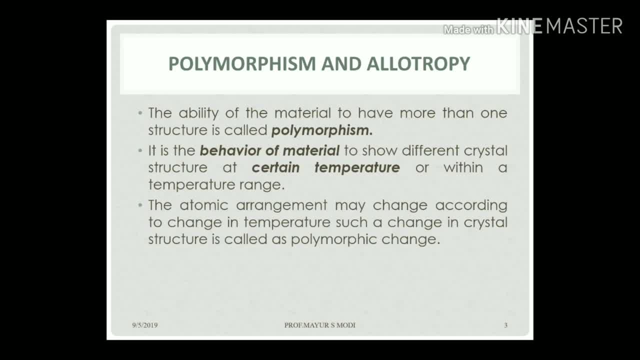 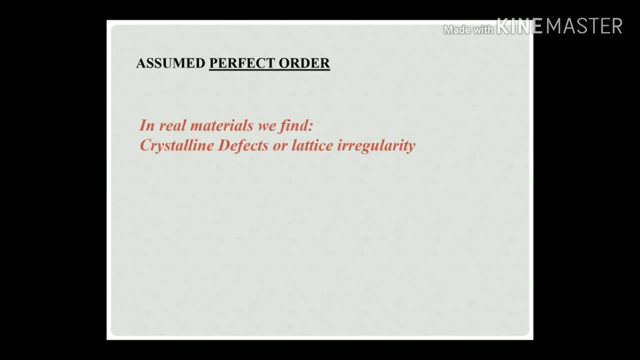 crystal structure is called as a polymorphic changes balls are about 30 эксп Cos enemies behind to choose material drawn from material. it will be cut into smaller pieces or round pieces that handle silicon. so the key required for this process are the ye'hee. let us assume that the perfect order structure for 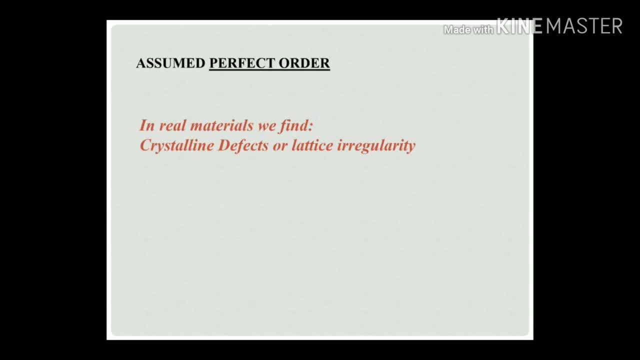 materials, but into real materials it will be the crystalline defects or laddice irregularities. so that is, regularity is presented into the structure by the atoms, не errors in the perfections, with dimensions on order of an atomic diameter to the many lattice sides. So just you can see any deviations from the perfect atomic arrangement in a crystal. 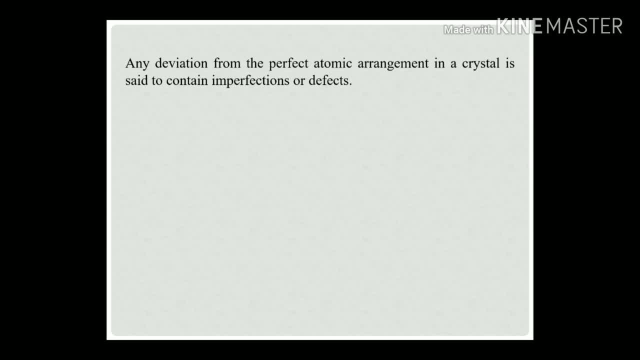 is said to contains imperfections or defects. So there are major four category of the crystalline defects. First, zero dimensional defects, or you can say the point defects occurring in a single lattice point One dimensional defect, linear defects, or you can also say the dislocations. 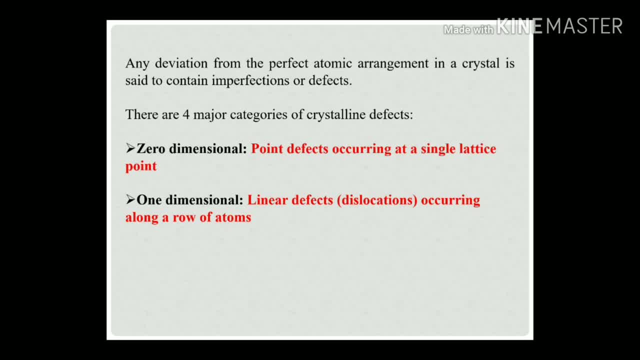 occurring along a row of atoms. Two dimensional defects, or you can say the planar defect, or surface defects occurring over a two dimensional surface in the crystal. Three dimensional defects, or you can say the volume defects, bulk void defects. So defects influences the electrical and the mechanical properties of the solid. by adding. 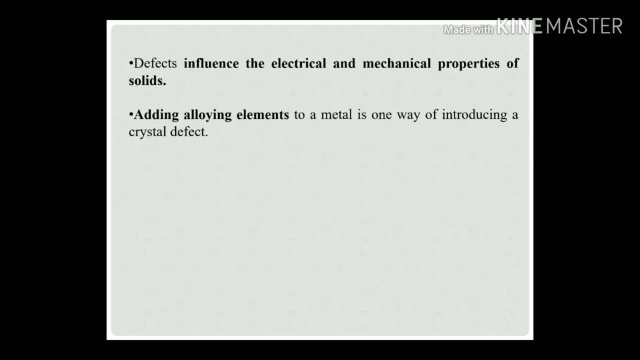 alloying element to a metal in one way to introducing a crystal defects, So crystal imperfection, have a strong influences upon many properties of the crystals, such as strength, electrical conductivity and the quality of the material. So the crystal defects are the most important properties of the material. Thus, some important properties of the crystals: 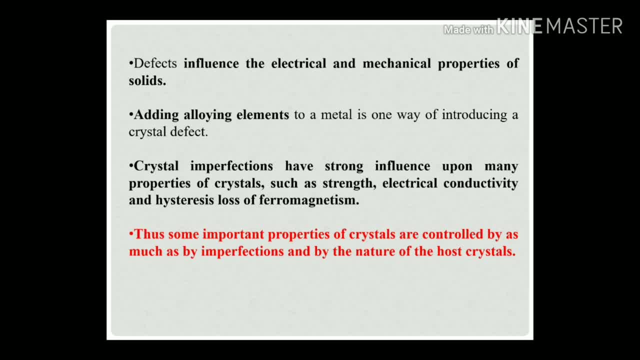 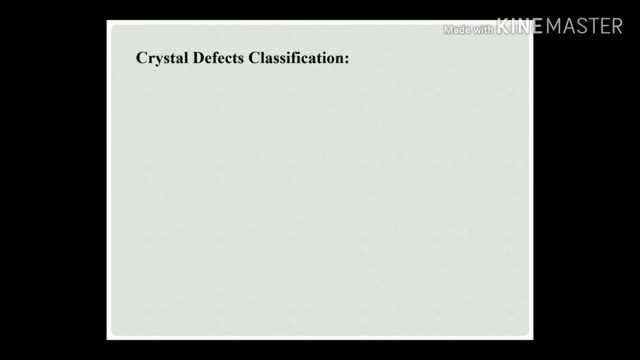 are controlled by as much as by imperfections and by the nature of the host crystal defects and its classifications. So based on to the point defects, or you can say the zero dimensional defects, vacancy kind of point defects, Schottky kind of point defects, self-interstitial kind of point defects, 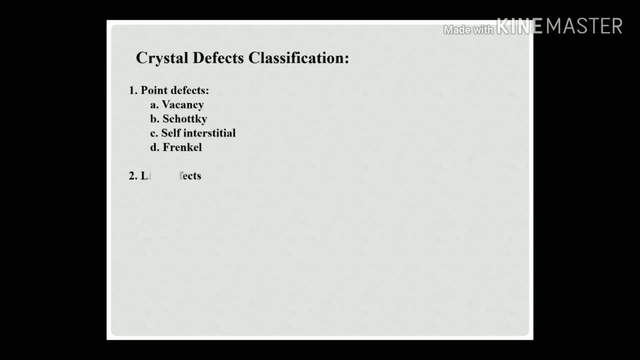 Frenkel kind of point defects in case of line defects, or you can say also a dislocation kind of defects. So edge dislocations, screw dislocations, surface defects, grain boundaries defects, tilt boundary defects, twin boundary defects, stocking fault kind of defects, volume defects, inclusions volume defects and so on. 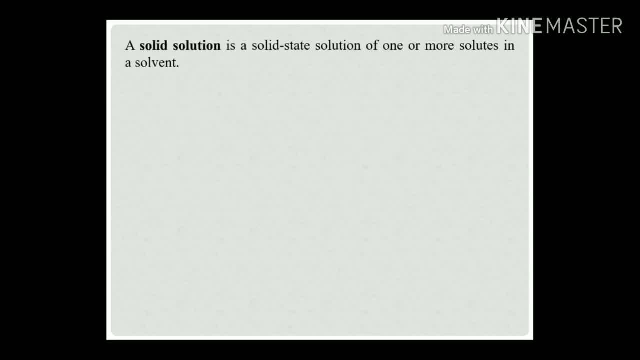 This will Allah Duhmani, and this will be that a small phenomenon will be already gone. So we have discussed about it. So right now I am actually going to discuss a 87 possessed metal in the prod contrat for a piece: 100 black and journalism gaan base, 22 gold. 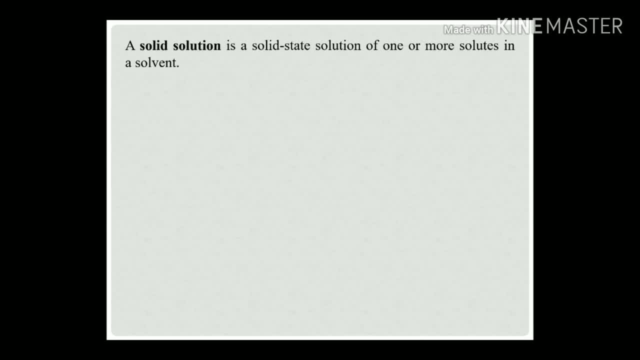 So this will be huge piece of metalstain primary material in a single top here in this. why? what so dining on man knowingly having K mått create their cat's material? So to measure all the time right now, to measure all the time. 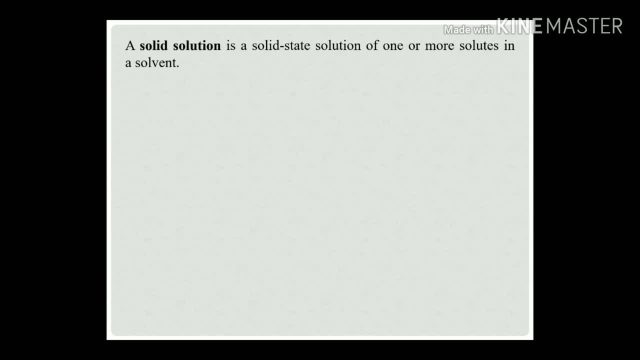 metal atoms, So solute metal atoms. it will be occupying the space into the solvent structure of the materials and to form the new materials. and that new materials it would be said to be a solid solution. So, as per the definitions, a solid solution is a solid state solution of one. 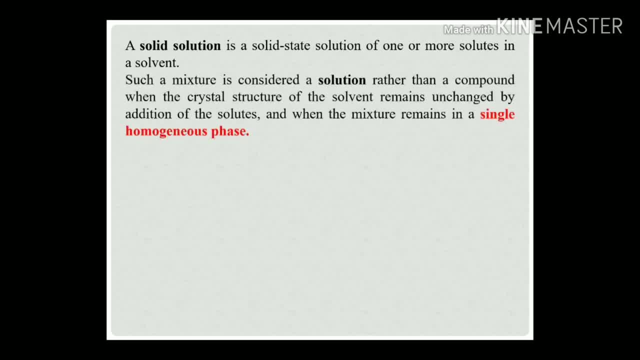 or more solutes into a solvent. Such a mixture is considered as a solution rather than a compound when the crystal structure of the solvent remains unchanged by the addition of the solutes and when mixer remains in a single homogeneous phase. So single homogeneous phase means it will be mixed. 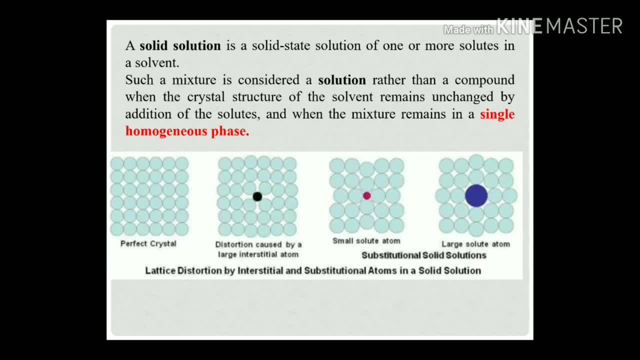 a single solid materials. So let us see the some of the examples. the first figure indicating the perfect structure, So you can considering it, will be the solvent structure. If there is a some alloying element will be added into the structure. so it will be changing a new structure, So new. 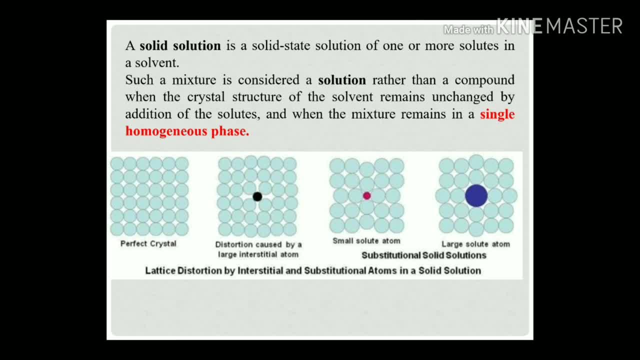 arrangement. you can consider it as a new structure. So you can consider it as a new structure, So can find so that new arrangement from the previous one that will be representing as a imperfections into structures, If it will be having the same size of atoms as we discussed for the solute and 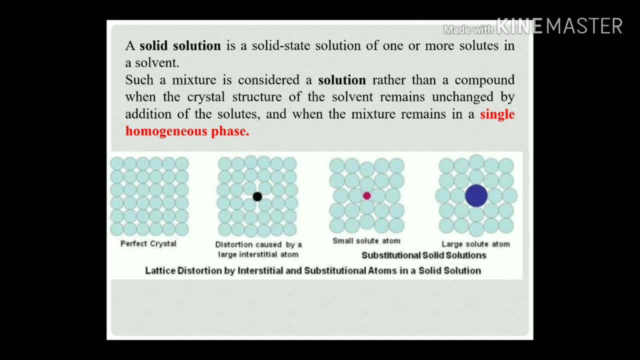 solvent, so that will be called as a substitutional kind of solid solutions. If it will be, the size is different for the solute and solvent, so that will becoming a interstitial kind of solid solutions. If the solute member having a solid solution, then it will be called as a substitutional kind of solid. 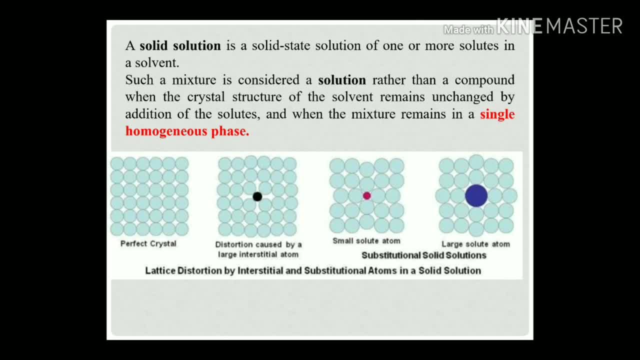 solutions. If it the 可以 have a smaller size, so that will be representing into the suppose in heated theed. on the smaller figure That will be representing small solute atoms. If the address it into a smaller size of the solute, it will be making a interstitcial solute solution. 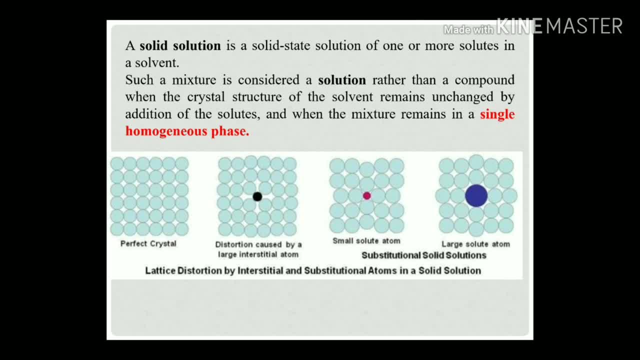 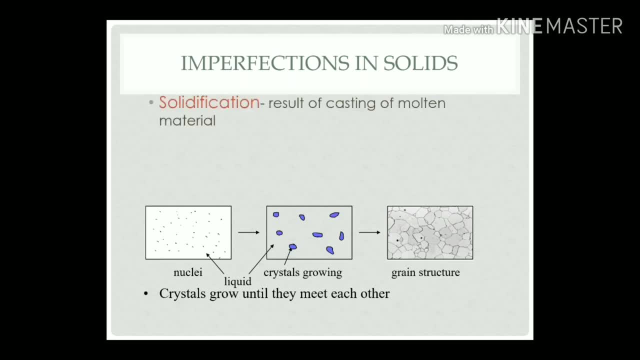 If the solid contact, if it will be having the same size, so that will be making a substitutional in Kombatapa Н, psychoigenics. or Then details, Most important theory, into the imperfections, into solids, and forget we are lipstick and a growth of a nuclei. so in the case of solidification process, result of casting, 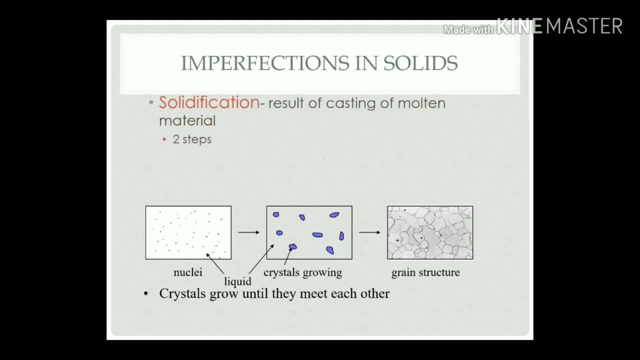 of the molten materials. it will be having two steps: nuclei formation and the nuclei grow to form the crystals and grain structure. you can see the initial positioning all the metal alloys that will be having a higher temperature into the liquid state. then you can carried out the solidification process. so 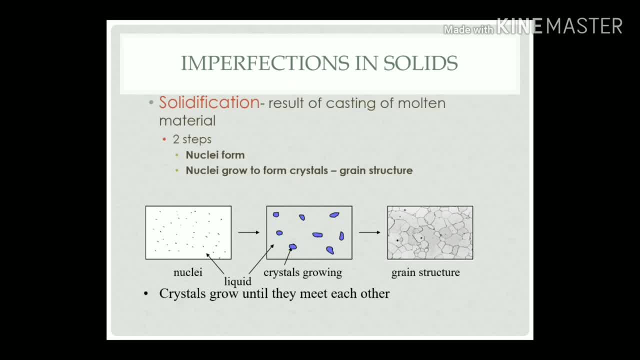 temperature drop down and some of the temperature, like the higher melting point of the metals, it will be considering as a starting point of the solidification in the case of binary alloy. so at initial state the nuclei formation. nuclei is nothing but the solid, tiny particles of either. 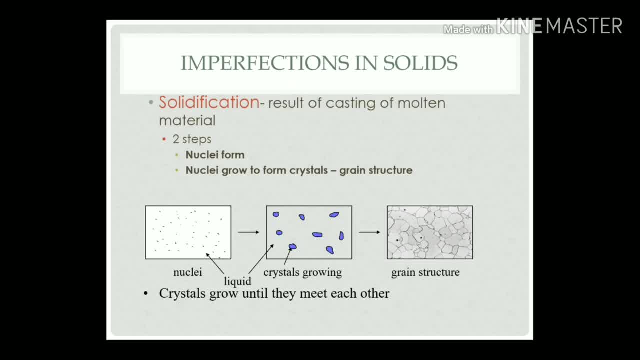 metal A or either metal B or you can say one of the metal. it will be having a solid, tiny particles and it will be representing by the nuclei. so after certain time of solidification process, that nuclei having a growth and finally it will be converting into grain structures. the crystals grow until they 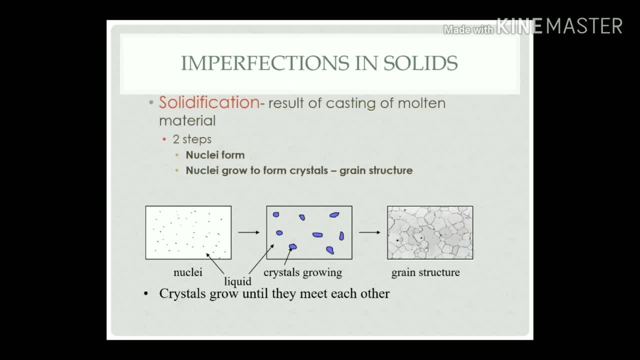 meet each other. so finally, one nuclei will be meet with the neighborhood nuclei and that neighborhood nuclei will be meet with their own neighborhood nuclei and it will be making a grain structure. so one grain size it will be differ from the another grains and that will be separated by the grain boundaries. 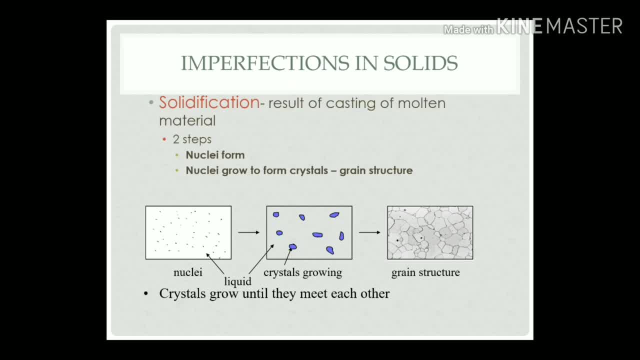 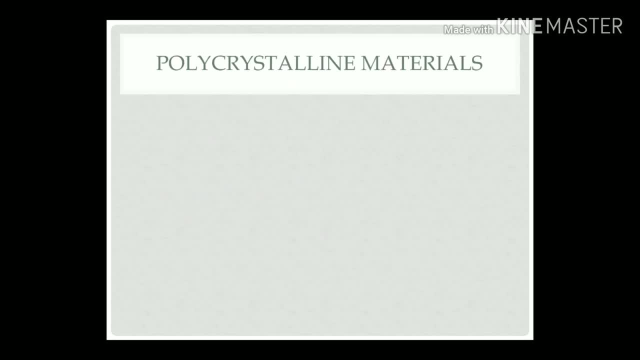 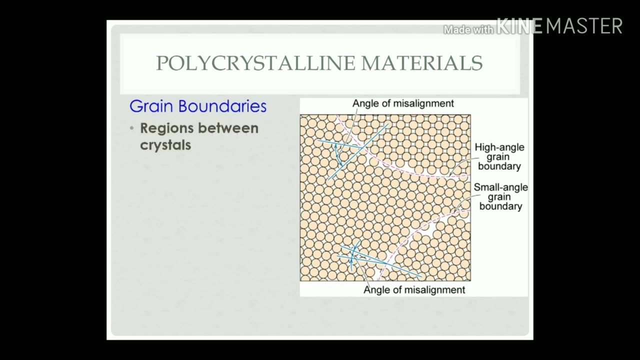 so, finally, you can get the structures in the form of grains and grain boundary. so start with a molten material. all are liquids, polycrystalline, what is just. you can see the structures. so grain boundaries, the region between the crystals, transition from one, from lattice of the one region to that of the others, slightly disorders. 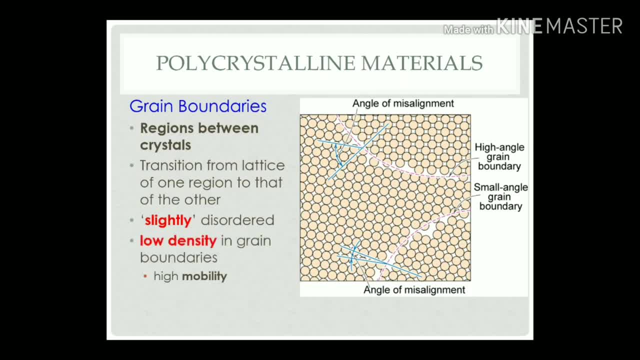 low density into grain boundaries. So low density it will be for the high mobility of the atoms, high diffusivity and high chemical reactivity. So here, just you can see the one grain size it will be differ from the another grain size with respect to the number of atoms. it will be present its direction, its basic structures. 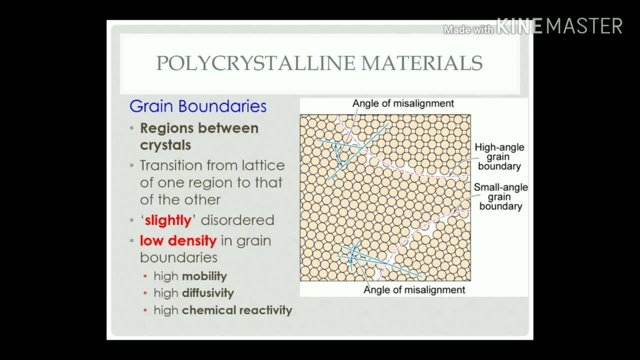 and occupying the space into the grains. So each and every grains it will be having a different angles. So it will be representing over here: small angle grain boundaries, high angle grain boundaries, angle of the misalignments, So some of the defects it will be present into the grains and grains boundaries. 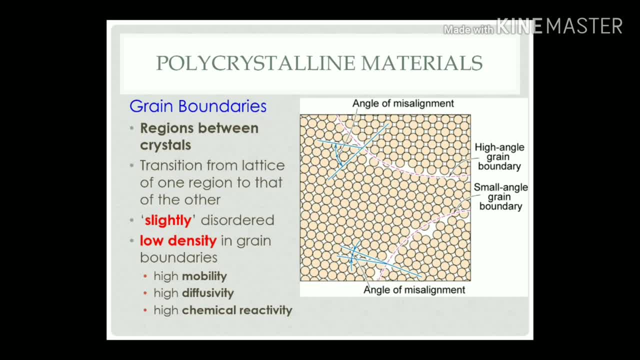 So that will be the representation of the polycrystalline materials. So finally, into the solidification process, your liquid, of your binary solid solution materials. it will be having a final structure in the form of grains and grain boundaries. So start with the defects, or you can say the imperfections the point, defects the point. 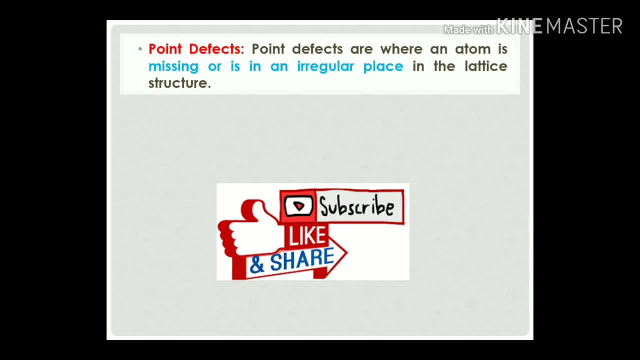 defects are where an atom is missing or is in an regular space into the lattice structure. Suppose, in the perfect order structure, one of the atoms. it will be permanently leaving their own positioning from the structures and it will be generating the vacancy. So vacancies. 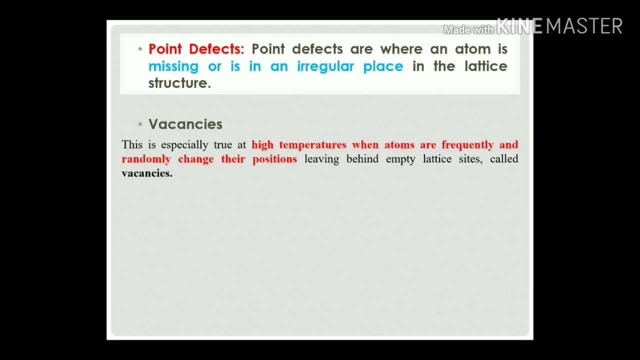 This is especially true at high temperatures, when atoms are frequently and randomly temperature armored, change their positions, leaving behind atoms lattice sites is called a vacancy, or you can see by different authors. vacancies are empty space where an atom should be but is missing. The higher is a temperature, more often atoms are jumping from one equilibrium position. 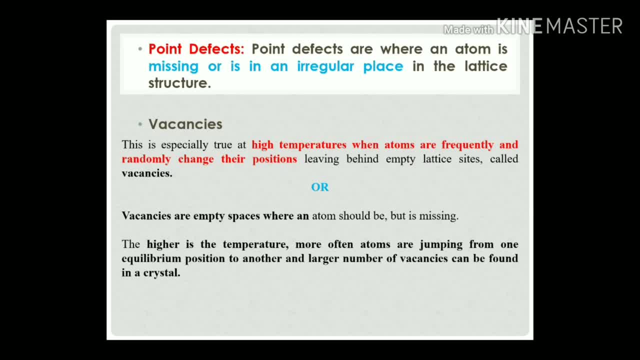 to another and large number of vacancy can be found into the crystals. So interstitials, or you can say the atoms that are squeezed in between regular lattice sites, if the interstitial atoms is of the same species as a lattice, atoms is called as a self interstitial. 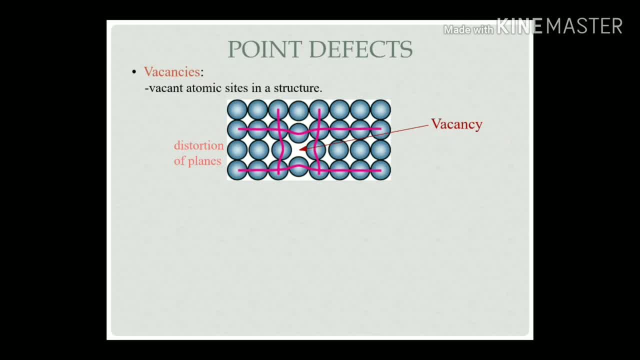 So here we are discussing with the vacancy kind of point defect. from the figure you can see that one atoms, it will be missing their own positions from the structures and it will be out of the structure. So by leaving their positions it will be generating the vacancy to such kind of defects. it will 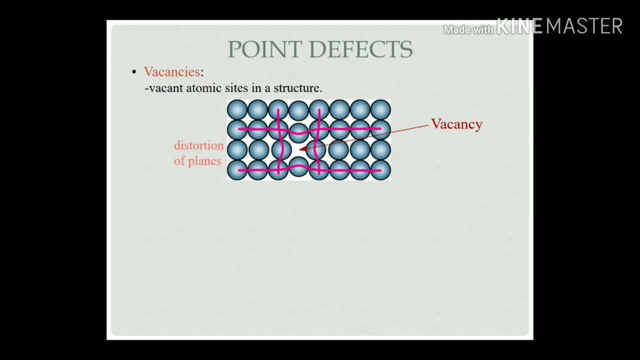 be present into the materials. it will be called as a vacancy kind of point. defects present into the structures. Second, one self interstitial, so one extra atoms it will be positioning in between. perfect order structures, says from the figure shows that one extra atoms it will be occupying. 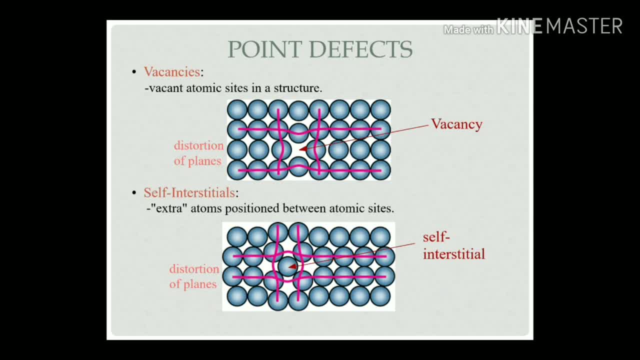 the space Into the perfect order structure and it will be also making a defects, or you can say the imperfections, into perfect order structure. that will be representing as a imperfections into solids and by the addition of the one extra atoms it will be called as a self interstitial. 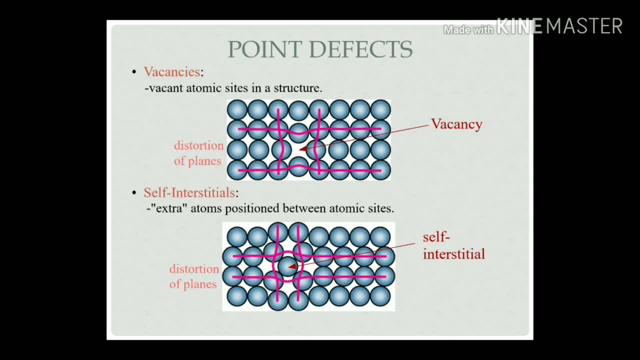 kind of point defects. So in case of vacancy, atoms are moving there, leaving their own positions, and in case of self interstitial, one extra atoms, it will be added into the structure. So by leaving there positions and by additions it always make the imperfections into structures. 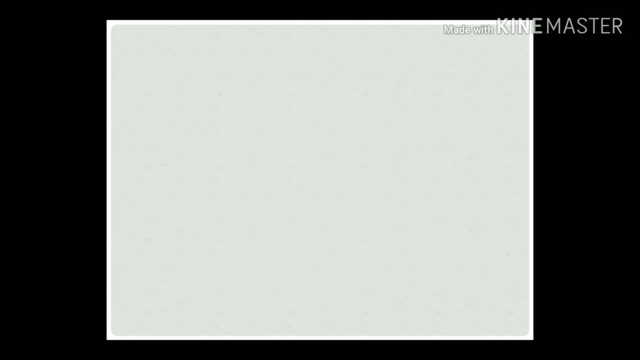 and that imperfection. it will be said to be a imperfection, or you can say the defects ø Short, key defects is a type of vacancy in which an atoms, being free from regular sites, migrates through a successive steps and eventually settles at the crystal surface. a pair of anion 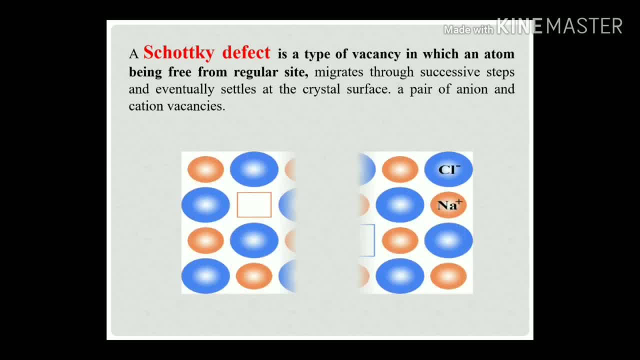 and cation vacancies Ò Ò Ò into the figure one positive ion and one negative ions. it will be leaving their own positions and it will be occupying the new positions at your boundary region. So always it will be in the pair of positive and negative ions from the structures. that will be called as a Schottky kind of. 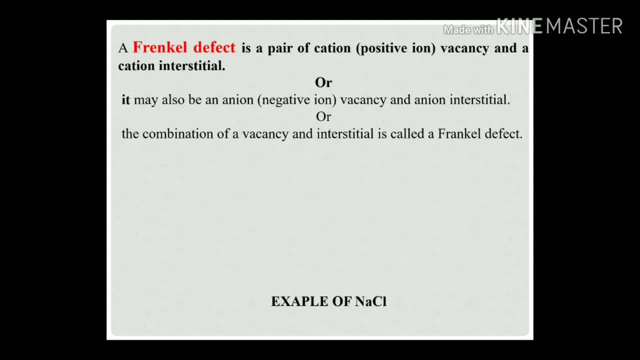 imperfections or defects. A Frankel defects is a pair of cation, or you can see the positive ions- vacancy and a cation interstitial, or it may be also be an negative mileage vacancy or anion interstitial. or you can say that the combination of vacancy and interstitial is called a Frankel. 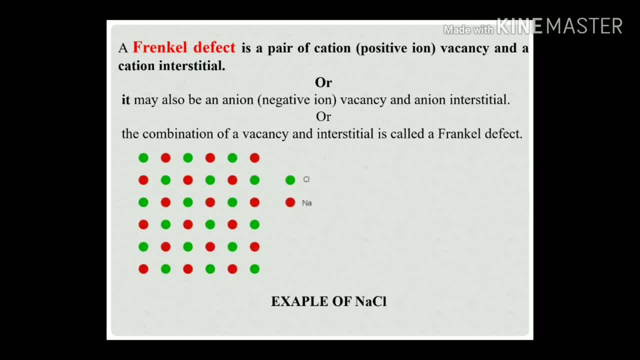 defect. So three definitions for Frankel defects. let us see with the some of the examples. Here is the perfect structure of NaNCl. So now you can see one positive and one negative. it will be leaving their own position from the structures and it will be occupying the new positions in between structures. 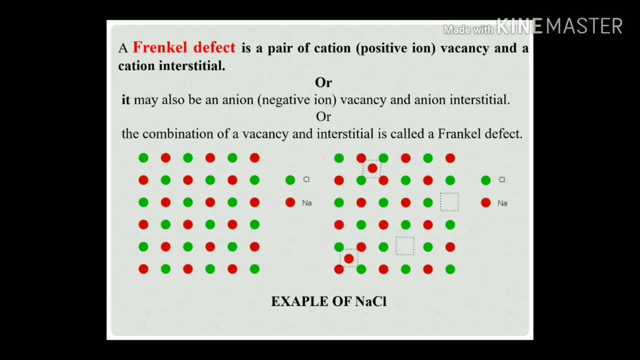 so by the leaving their own positions it will be generating the vacancy kind of point defects and by occupying the new space into the structure, so that will be the interstitial kind of point defects. so you can see that it will be the combination of vacancy and interstitial kind of 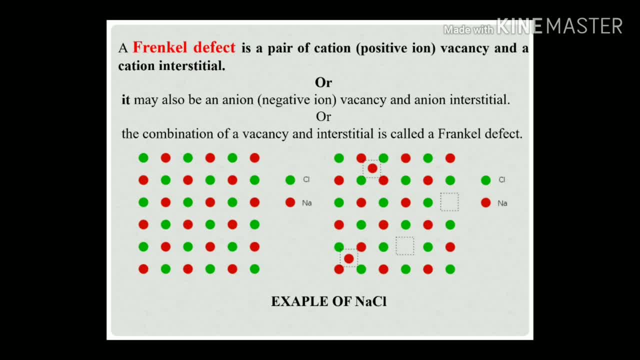 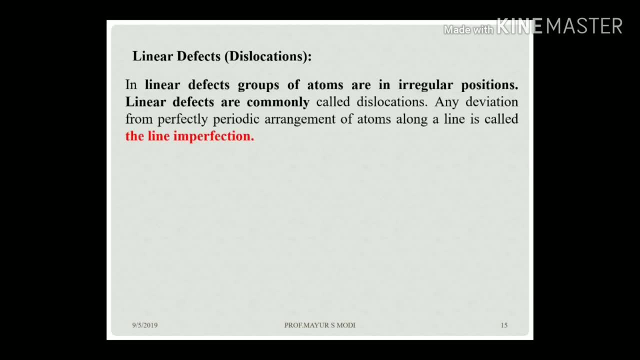 point defects and that will be your frankel defects. line defects or you can say the dislocations in linear defects group of the atoms are in a regular irregular positions. linear defects are commonly called as a dislocations. any deviation from the perfect periodic arrangement of the atoms along a line is called the line imperfections. 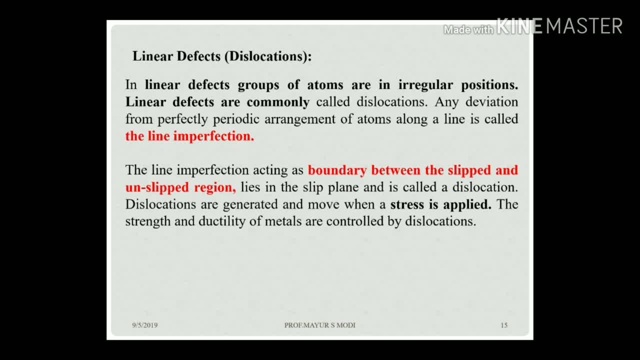 so the line imperfection acting as a boundary between the slipped and unslipped regions lies in the slip plane is called the line imperfections or disc dislocation. disc dislocation are generated and moved when stress is applied. the strain and ductility of the metals are controlled by the dislocation. 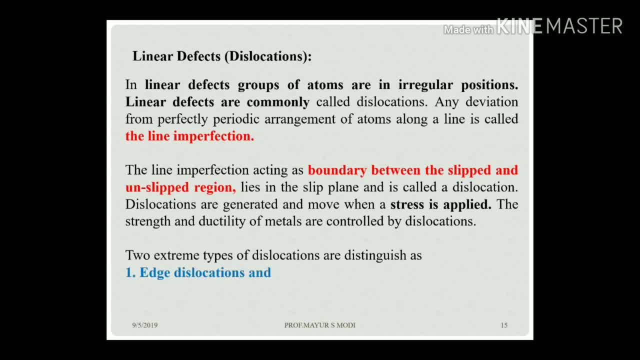 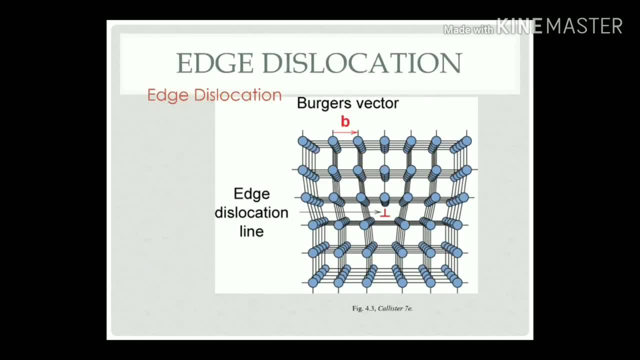 there are entirely two types of dislocation: is dislocations and screw. dislocation: ogy, Demon, the Alien. dislocations from the figure: the above portion, it will be having a perfect structure and below portion, it will be having perfect structure. line Tor r will be this websites. 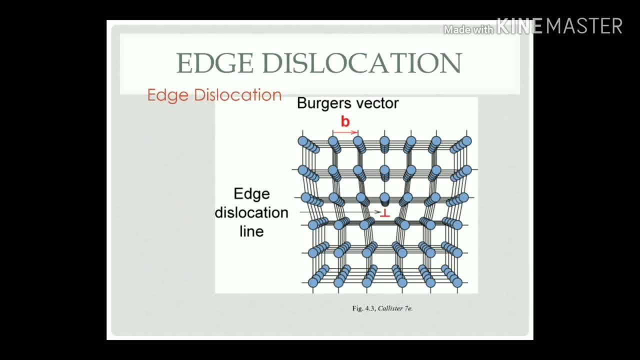 units, the of the one extra line of the atoms, and so it will be dividing into two parts: slip region, so above portion and below portion, or you can say slip region and unslip regions. so after applying the stress, or you can see the shear stresses, that line of the atoms, it will be moving. 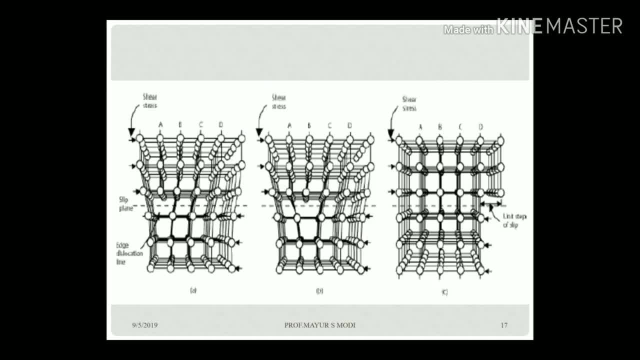 into the structure. let's see with the another figures here. it will be the one extra line of the atoms a that will be added into the structure and it will be having a line kind of dislocations. so above portion from the slip lines it will be a slip region and unslip regions. so after applying the shear stress from 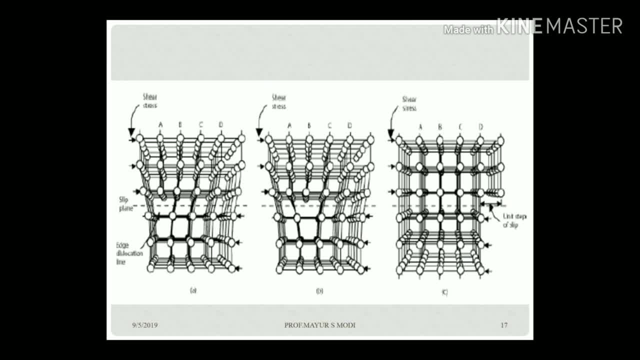 the both the end, on your slip and unslip regions, that extra line of the atoms a, it will be try to jumping over a, b, and try to jumping over a, c, and finally you can see that it will be one of the edge of the structures. that's why it will be called as a. 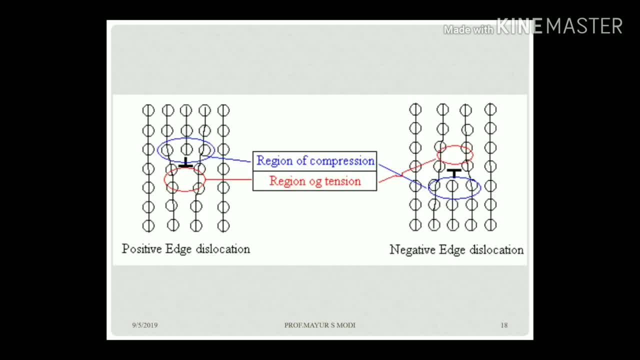 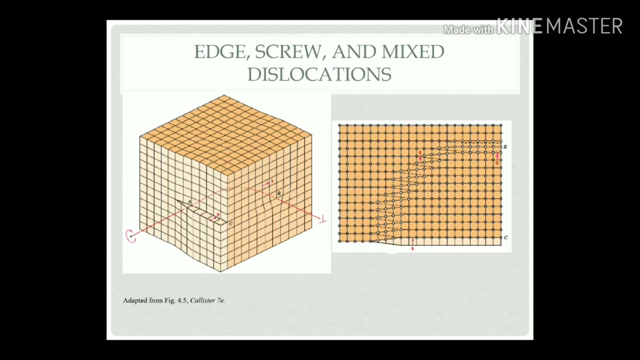 kind of dislocations. You can see that if the one extra line of the atoms it will be added into the top positions, that will be considered as a positive dislocations. If it will be find at the bottom of the structure, so it will be called as a negative edge dislocations, Screw dislocations, So just 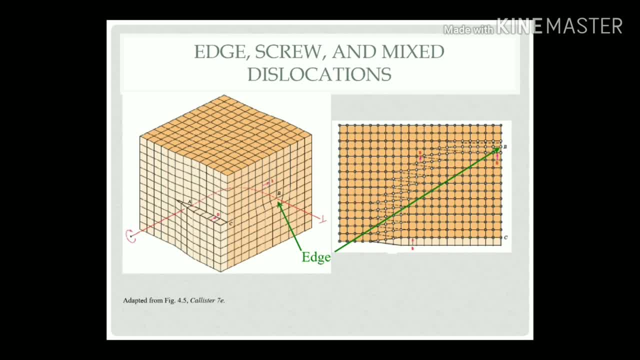 you can apply if the edge dislocation, it will be present into the structures and you can apply the torsional effect so it will be moving in, like into the figures. So basically, Burgers vector, that will be the distance, it will be measured from one atom to another atoms. if the line dislocations, it will be the presence in. 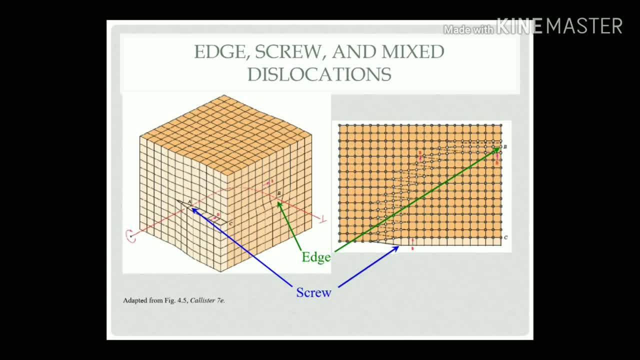 case of edge dislocation, it will be the perpendicular to the dislocation line. In case of screw dislocations, it will be the parallel to the dislocations line. If the both are present, or you can say your component, it will be subject to the torsional as well as your shear stress. So it will be. 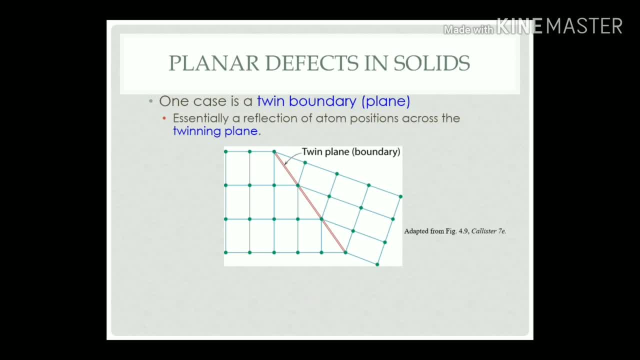 having a mixed kind of dislocations, Planner defects into the solids. Suppose the top surface of your structure it will be get damaged at certain angle So that boundary it will be twin boundary kind of defects you can see into the structures The essentially the reflection. 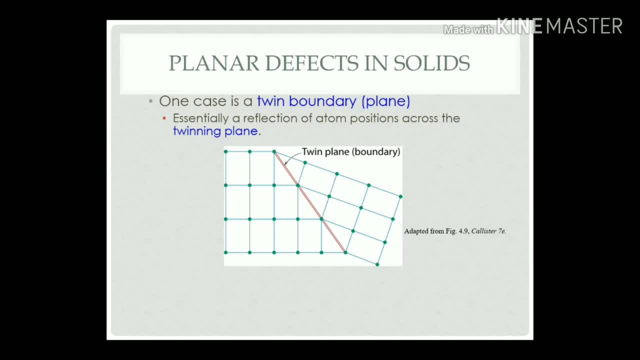 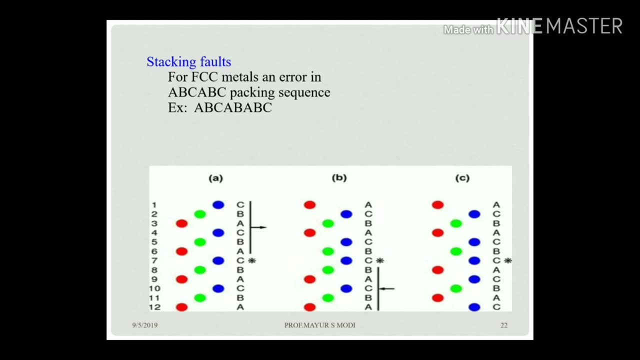 of the atoms positions across the twinning plane, Stocking foil kind of defect. For a perfect structure it will be having A, B, C, A, B C kind of sequence. but if you find A, B, C, A, B C and B C, So there is aließen here, So the alkaline equivalent to that, the top of the dielo wall.